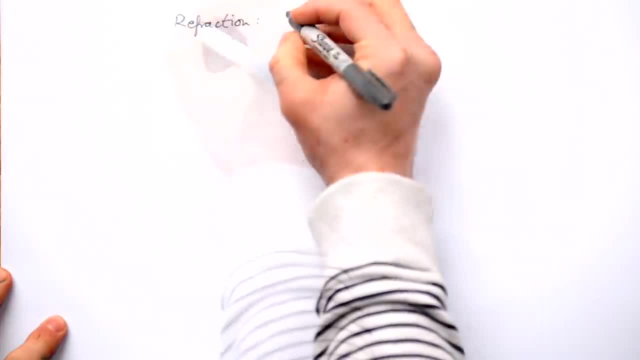 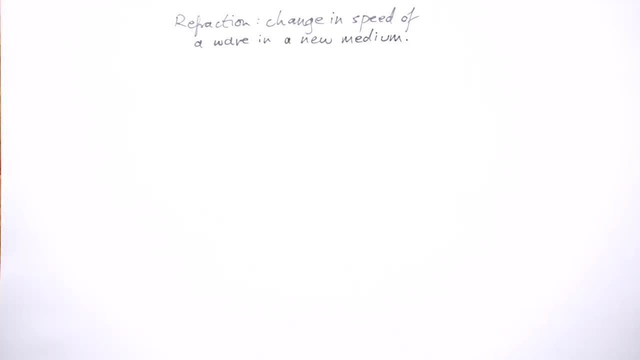 All right, let's talk about refraction Now. refraction is the changing of speed of a wave in a new medium. What does medium mean? Well, medium just means the thing that the wave is traveling in. So for sound, the medium could be air, it could be water, it could be a solid as. 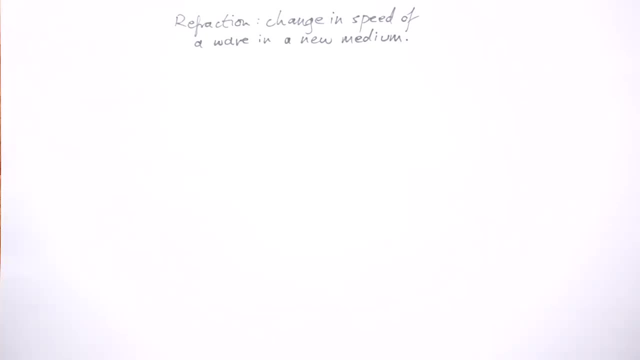 well, which begs the question: what's the medium for light? Well, people used to think that there was a physical medium called the ether, but that was quickly dismissed. If you want to know all about that, then have a look at the Michelson-Morley experiment. You could say that the medium for 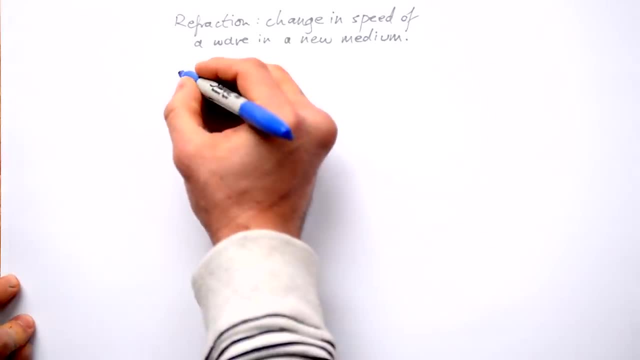 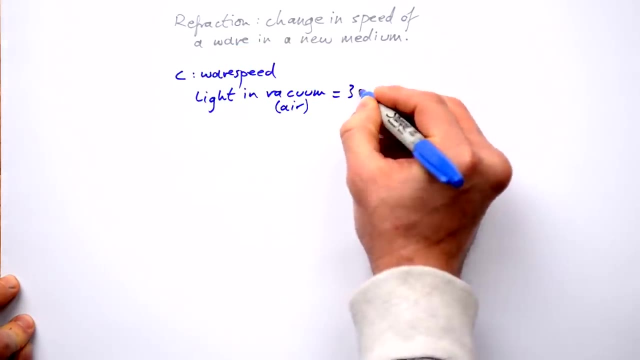 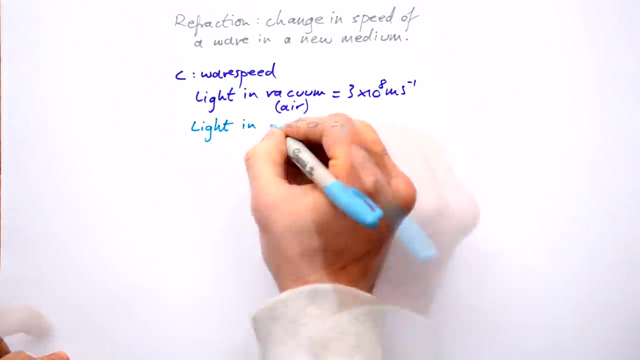 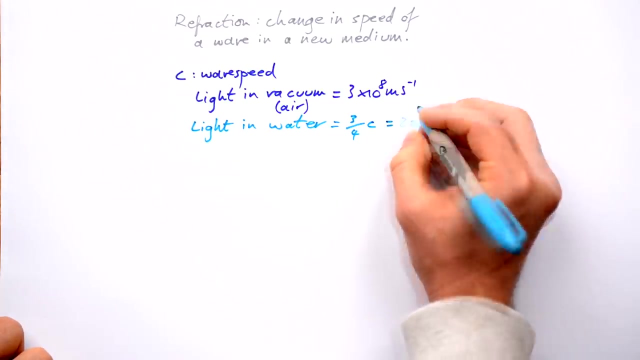 light is space itself. Now we give the symbol C for the speed of a wave. Light in a vacuum is very similar for air as well- is three times 10 to the eight meters per second. Light in water, however, travels at about three quarters the speed of light in a vacuum. That's about two. 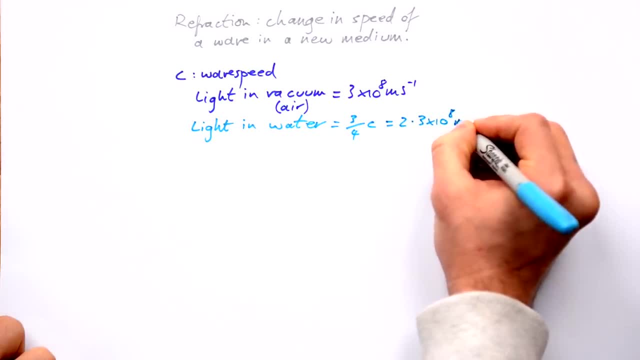 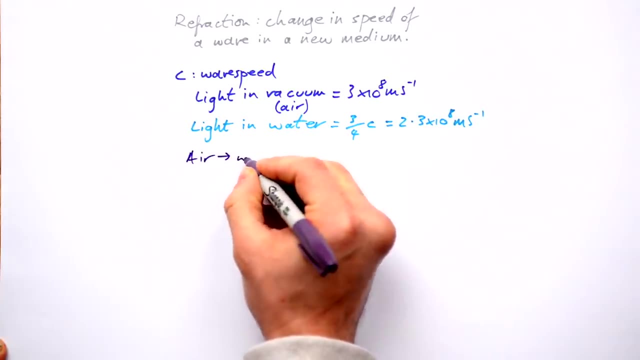 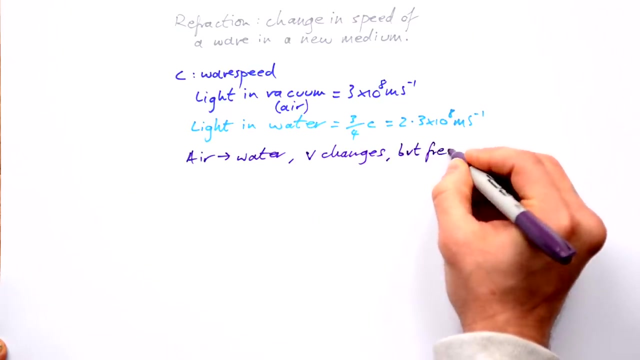 point three times 10 to the eight meters per second. So quite a big difference. When light goes from air to water, the speed changes. Now I'm going to call the speed V here, because I'm going to reserve C for the speed of light in a vacuum, But the frequency stays the same. 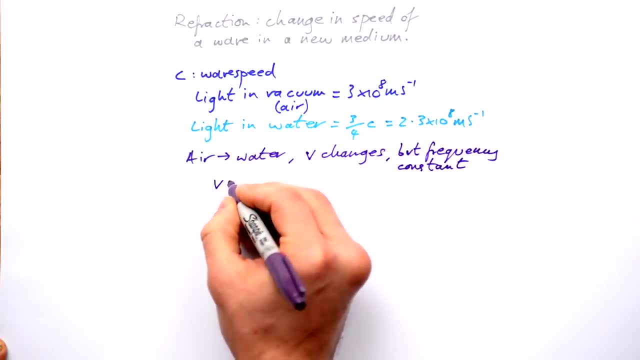 That's kind of weird, isn't it? What's our wave equation? V equals F lambda. If the speed goes down as it goes into water, but the frequency stays the same, then that must mean that the wavelength has to go down as well, because, as we know, that the velocity therefore has to be. 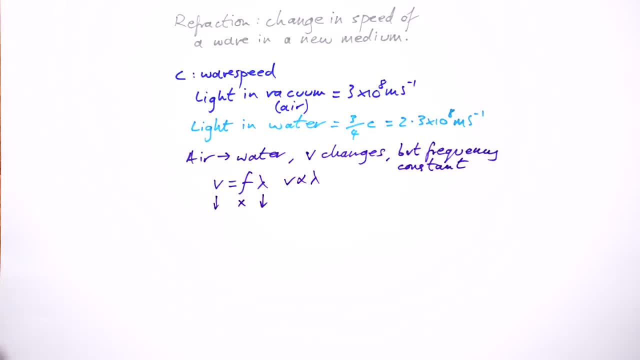 proportional to the wavelength. Whatever one does, the other one does as well. So what does it look like? Here's our air, Here's our water, Here's our boundary in between. So we've got a wave between. Light comes in, And as it hits the water, the waves start to bunch up. As it goes that way, 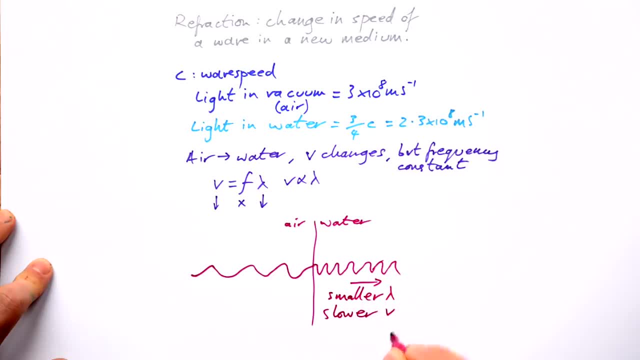 smaller wavelength, slower velocity. If the light comes head on, that is, 90 degrees to the boundary, then the wave will just carry on going in a straight line. It's just that the wavelength we've got smaller and it will go slower as well. 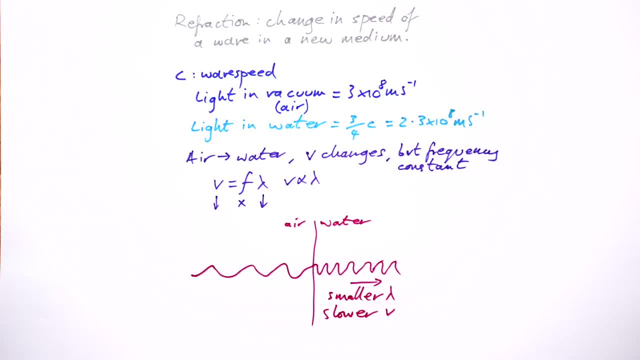 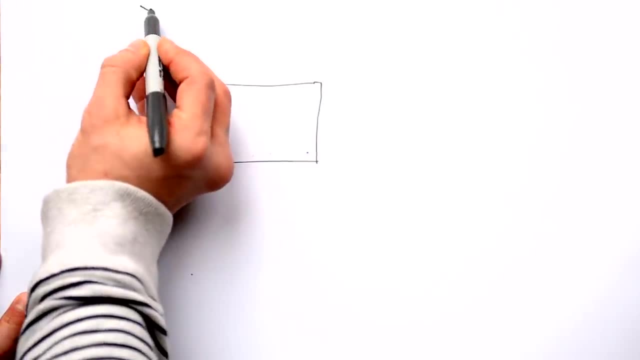 But what happens if the light comes in at an angle? That's when the really interesting stuff happens. Let's say I had a block of perspex or glass or something like that. Now the light is going to come from this direction here. We know that light. 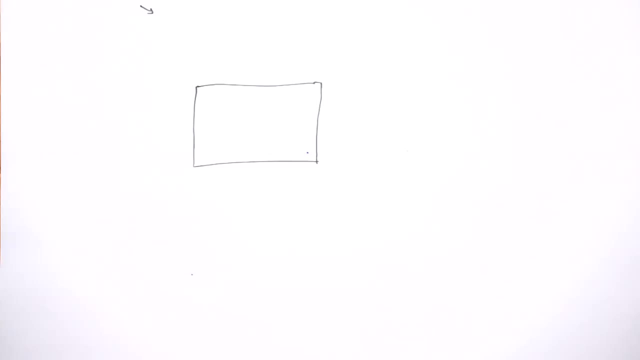 acts like a wave as well as just a particle going from A to B. So let's draw some wave fronts. We're looking down on the wave and these lines represent the peaks of the waves And they're coming in towards the bottom of the wave. 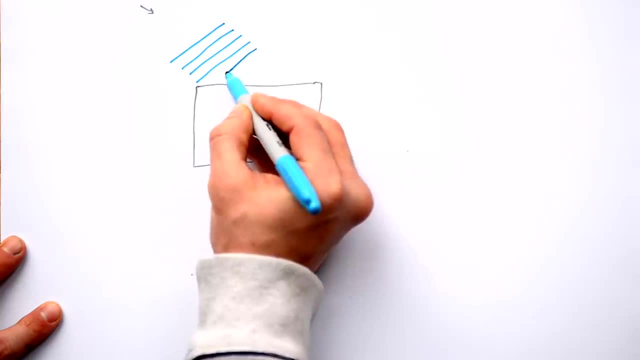 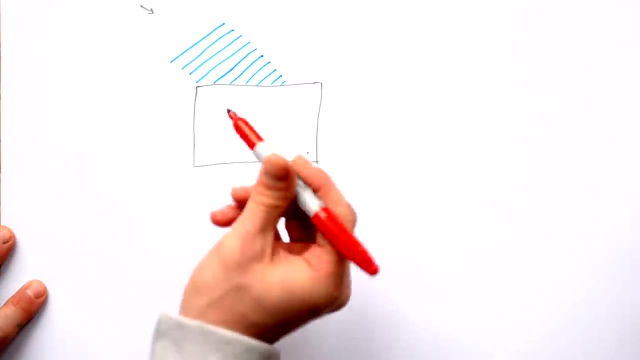 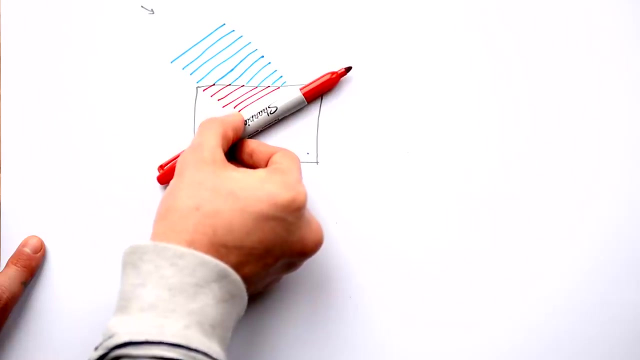 And the bottom of the wave is going to be the top of this block. In other words, they're incident on this block, But once the wave reaches the block there, a bit of the wavefront actually changes angle. So the waves come in like this, but then as they start entering the block, 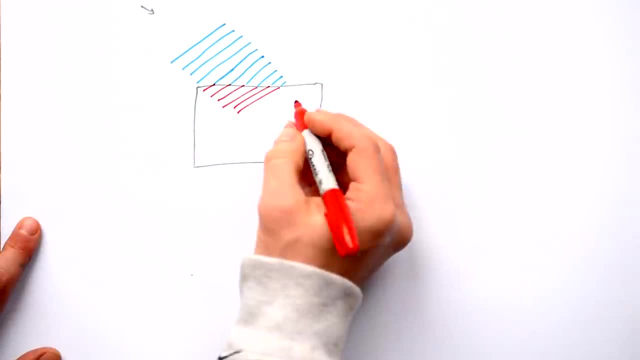 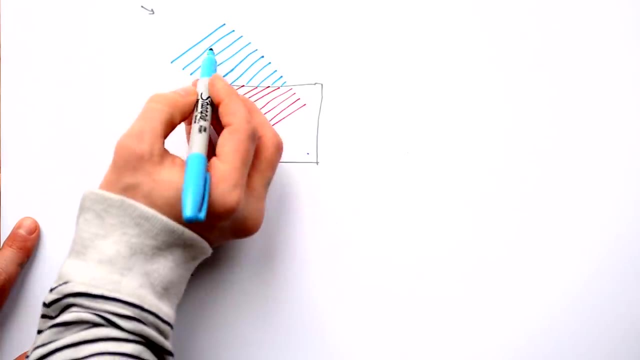 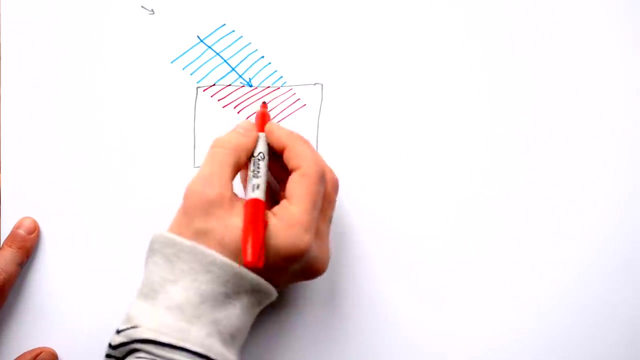 they turn and we can see that the wavelength has shortened in. it carries on like that. if i was to draw arrows showing the direction of the wave and where it goes. there's my direction of the wave going in and then here's my direction of the wave. 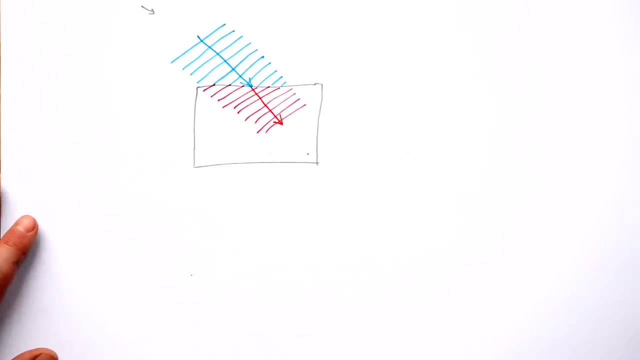 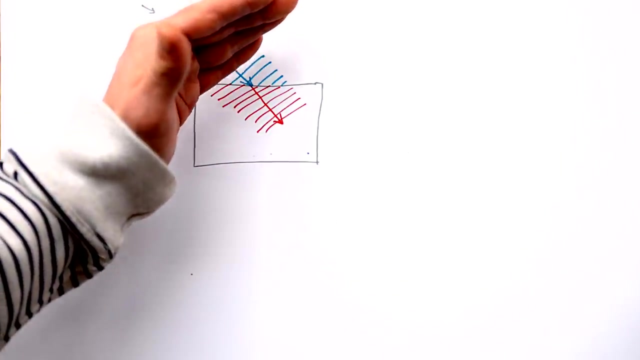 coming out, we can see that it's actually changed direction ever so slightly, but it has. this happens because a bit of the wave front starts slowing down before the rest of the wave front and so effectively drags the wave front round like that as it goes in. you can think about it like this: if 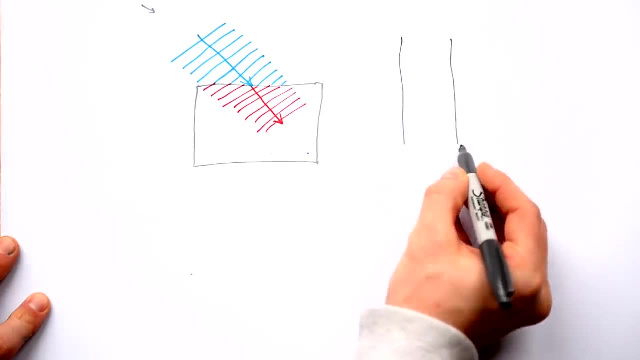 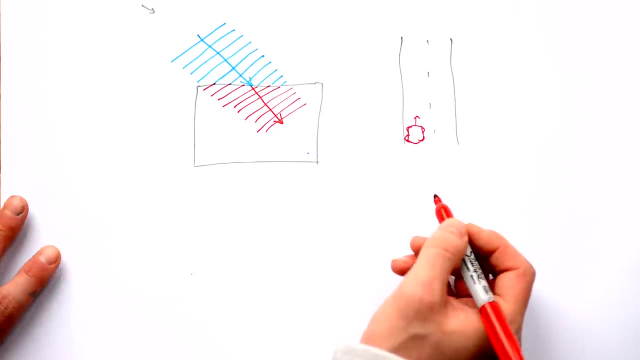 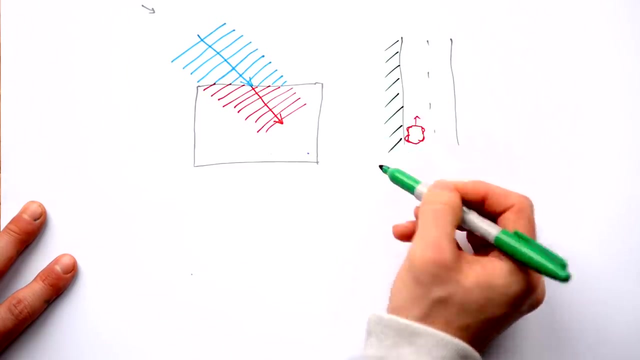 we have a car going along the road. so here's the car going along the road. we're looking down on the car. there's his four wheels and the driver starts to drop off, starts to veer ever so slightly towards the soft verge where this grass. what happens? we end up with the car's left wheels on the grass. 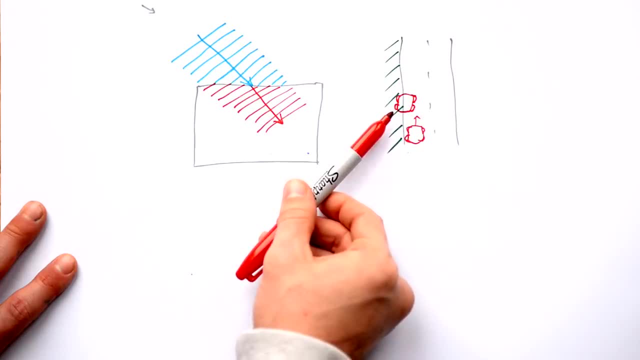 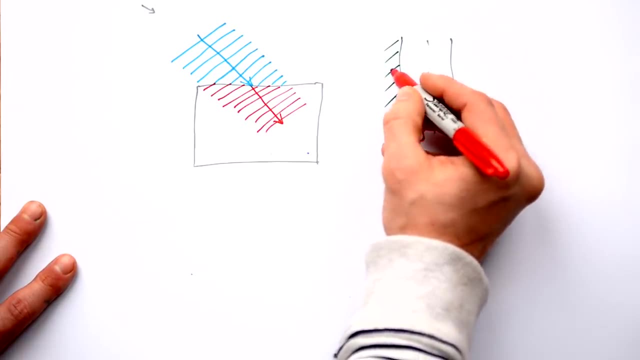 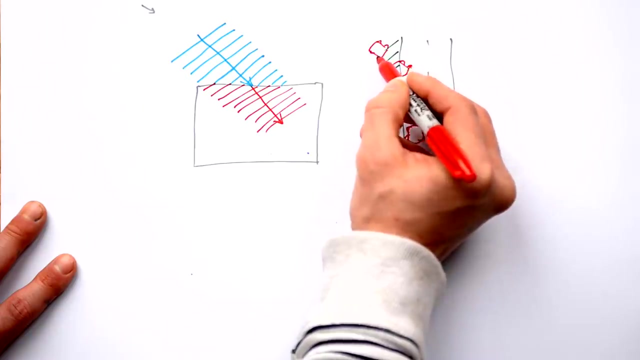 the right wheel still on the road. the left wheels they will skid. there's less friction. so that means the left hand side of the car will be going slower than the right hand side and it ends up turning. once it's all the way in it will just carry on going in that direction because all four wheels 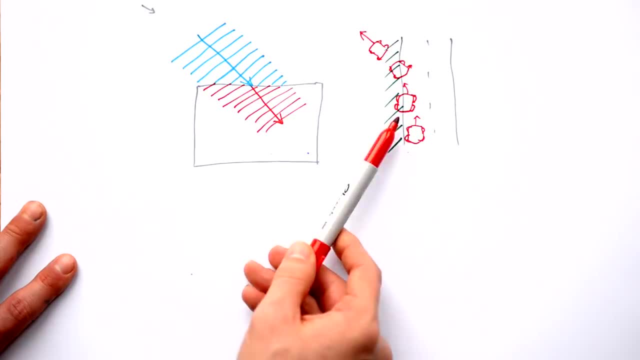 are going at the same speed, so we can think about refraction in these terms. part of the car is slowing down before the other part of the car, so it turns same thing with our wave fronts. luckily though, we do have a little bit of a difference between the left and the right side of the car. 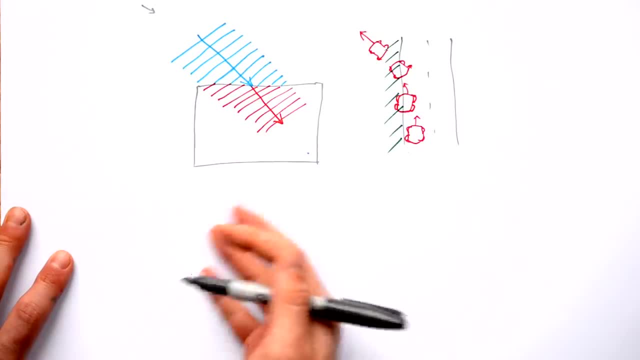 we do not have to draw wayfronts or cars every time we talk about refraction. so here's my air glass boundary and here is my ray of light coming in. we don't have to draw the wave fronts because this is just a very narrow ray of light. 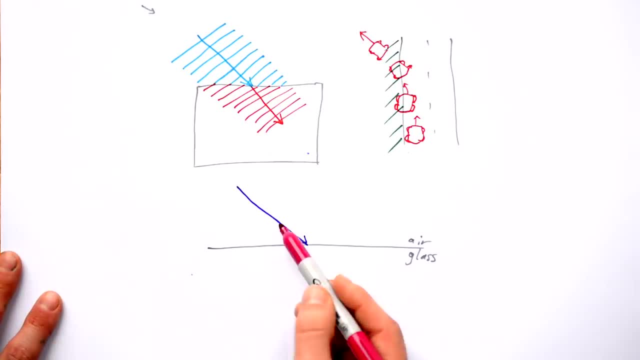 what angle is this ray of light hitting the glass at? we could give this angle here, but that's not as useful as what we actually do. what we do is draw a line that is 90 degrees the boundary, and that's what we call the normal. anything that's normal is 90. 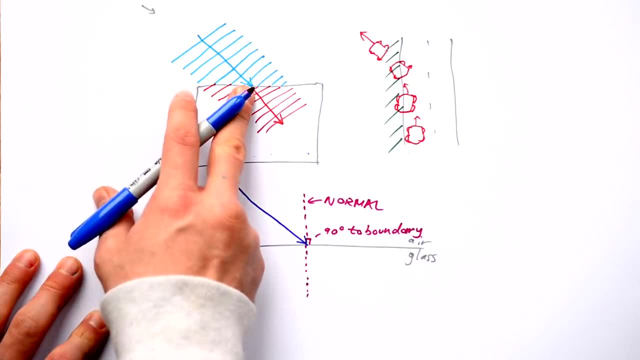 degrees to something. so we saw that if the light ray slows down as it goes into a new medium, then we can see that if we had a normal on here, we can see that bending towards the normal, like so the normal is what we measure all our angles. 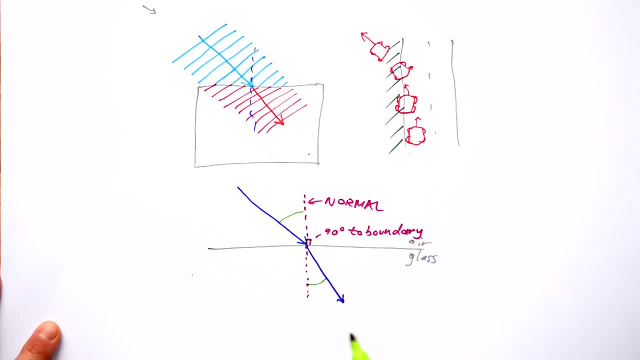 from. so we measure that angle and then we measure that, and we never measure the angle between the boundary and the ray of light itself. we're gonna call this angle here theta 1 and theta 2. we could also call them I and ah, whatever you want to call them: I and theta 1. 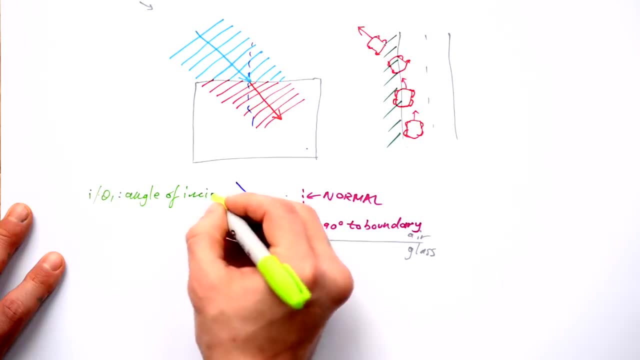 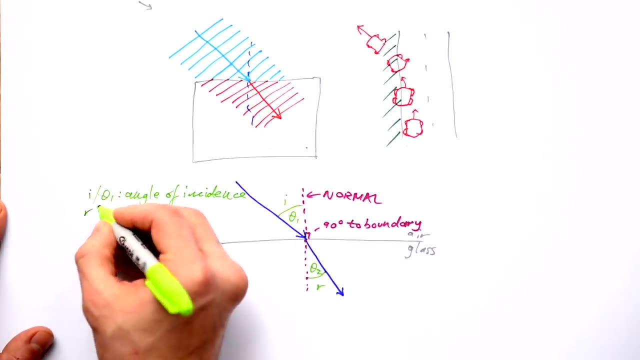 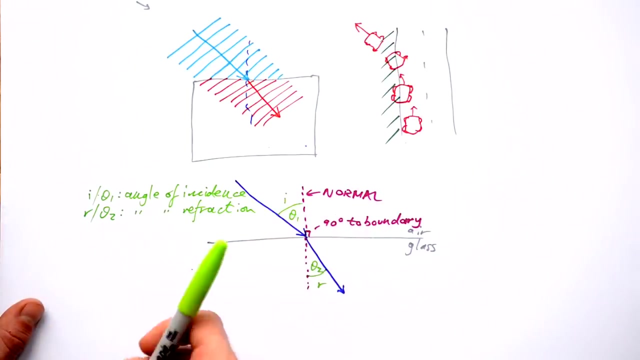 represent the angle of incidence. what angle the light ray is hitting the material at the new medium, at, and R theta 2 is the angle of refraction. so we said earlier the refraction is a change in speed of a wave in a new medium. generally, when we talk about refraction we talk about that happening, which 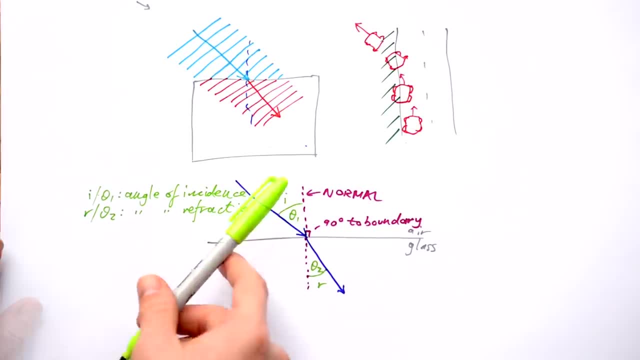 results in a change of direction of the wave. so this light ray here has been refracted. If it was going along the normal then it would slow down, but it wouldn't be refracted because it hasn't changed direction. As per usual. we need some way to quantify. 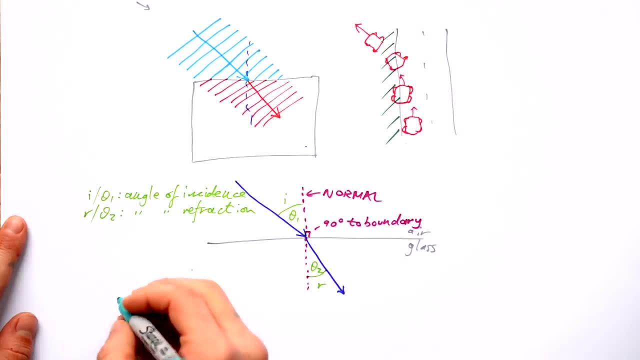 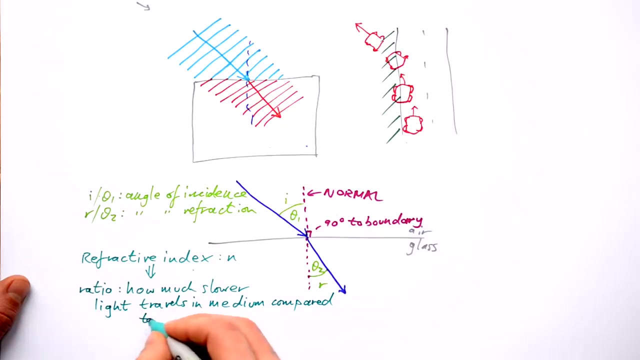 the change in direction that's happening here. This is done with something called refractive index And we give it the letter N. All the refractive index is. it's a ratio that tells you how much slower light travels in a medium compared to vacuum or air. 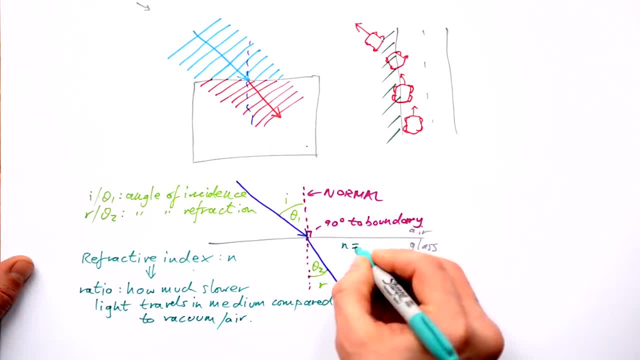 So I can tell you that for glass, the refractive index is 1.5.. All this means is that light travels 1.5 times slower in glass than it does in air. So we could say that the speed in the glass is equals to three times 10, to the eight divided by 1.5,. 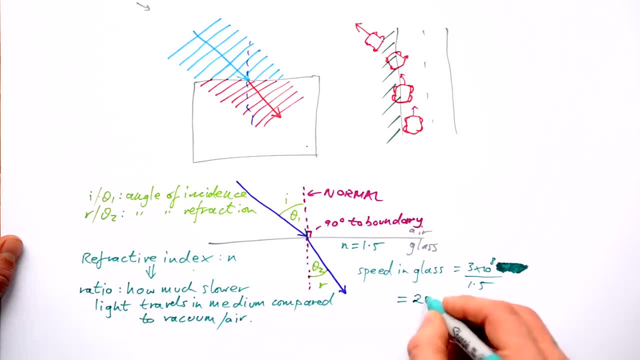 and that gives us a speed of two times 10 to the eight meters per second. That's all that refractive index tells you. It has no units because it's just a ratio, So a quick and easy way to remember what a high refractive index tells you. 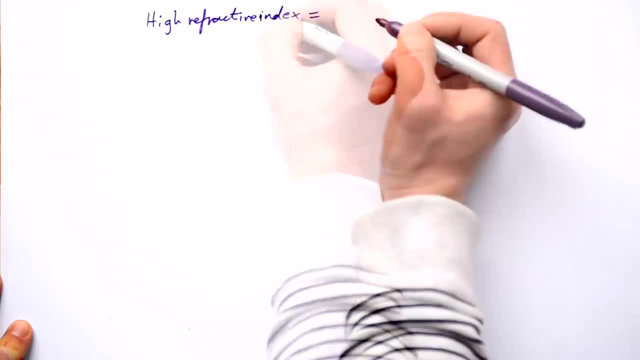 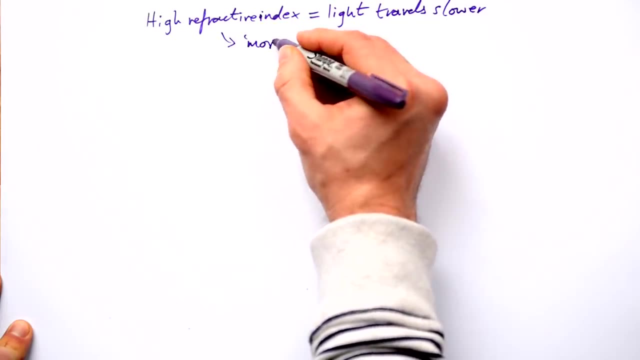 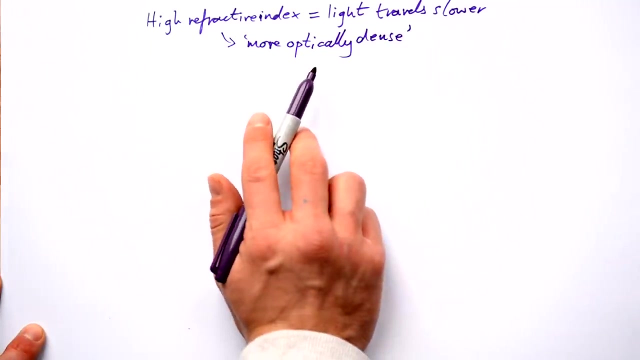 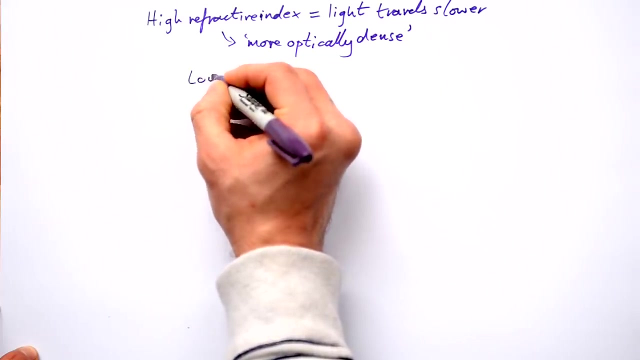 High refractive index or higher refractive index means that light travels slower and we can also call it more optically dense. More optically dense, so it's harder for light to travel through it, as it were. If light goes from a low refractive index. 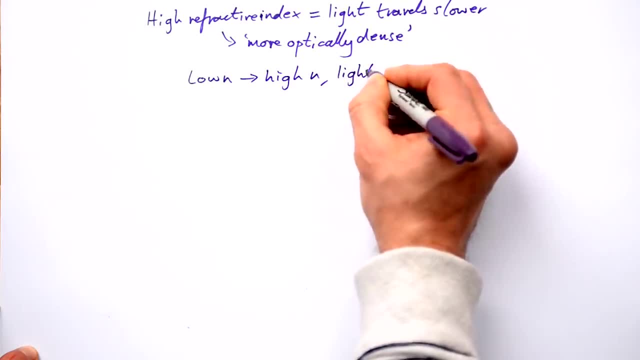 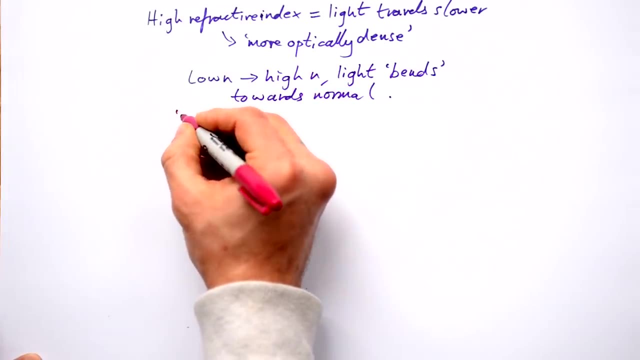 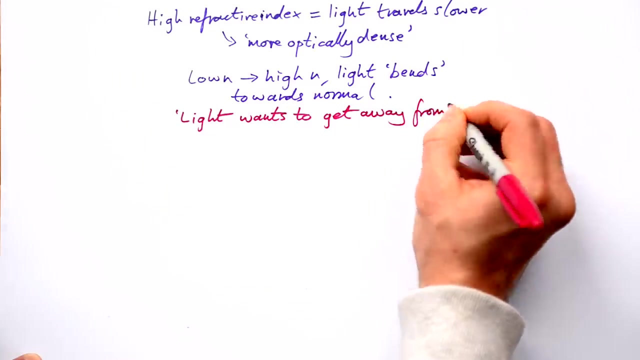 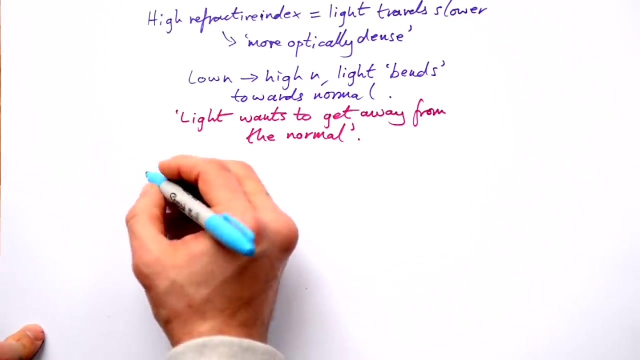 to a high refractive index. then the light bends towards the normal. Crude way of remembering it is. light wants to get away from the normal. The faster light can travel, the easier it is for it to get away from the normal. So you might see the equation written like this: 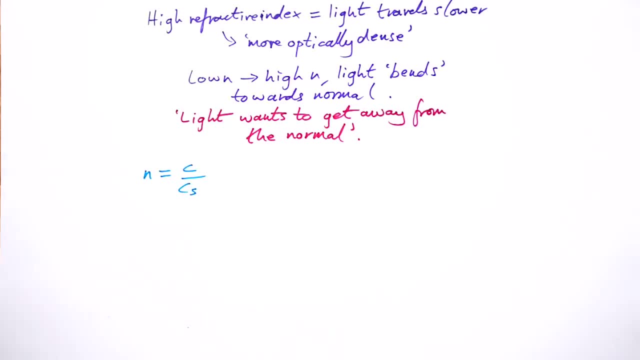 N equals C over CS And as refractive index this is speed in a vacuum Three times 10 to the eight meters per second. This is speed in the medium, But obviously this only works for vacuum or air into another medium. 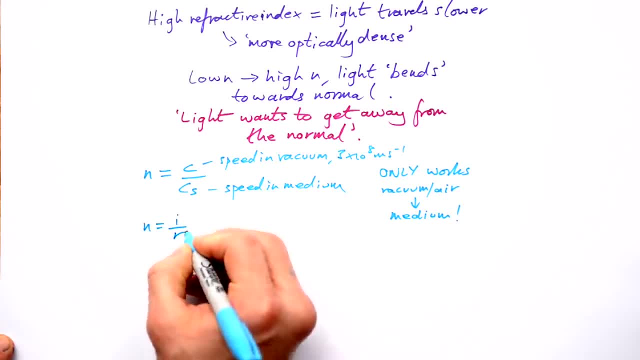 How do we get refractive index, though from angles, then Could we say that this is the case, Because we know that the smaller the refracted angle, the bigger the refractive index is going to be, So that means it's more optically dense. 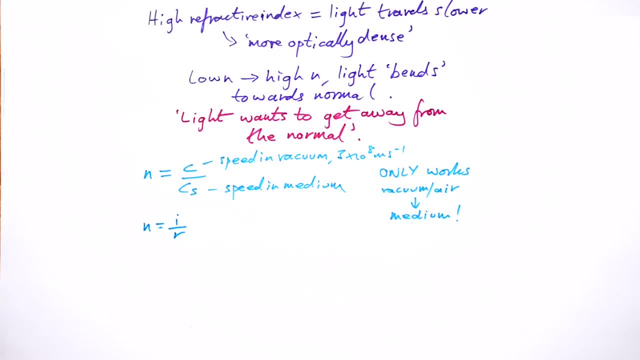 but it doesn't work. That doesn't give us the right answer. What does The sine of the angle, sine I over sine R, or we could call that sine theta one over sine theta two? By the way, if you test a material sending light in? 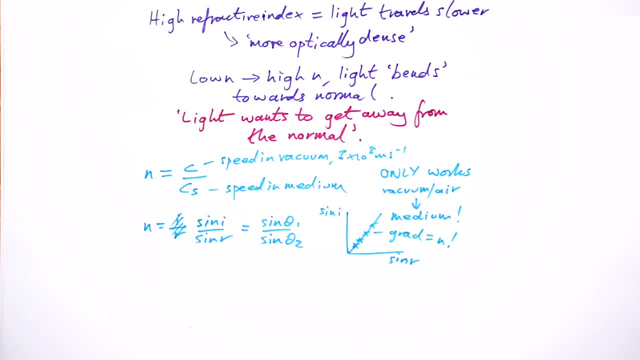 at different angles, you get a nice straight line. If you plot sine I against sine R and the gradient gives you the refractive index of that medium. What if we had light going from glass into water or vice versa, or light travelling between any two media? 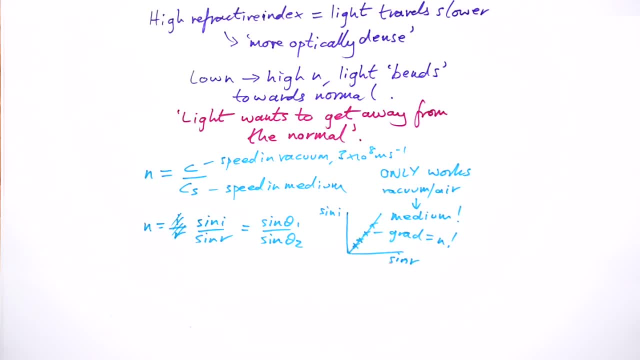 or mediums that aren't air or a vacuum. So we need a more general equation. So what is the refractive index for air? Well, it's going to be one, because three times 10 to the eight, divided by three times 10 to the eight, is gonna be one. 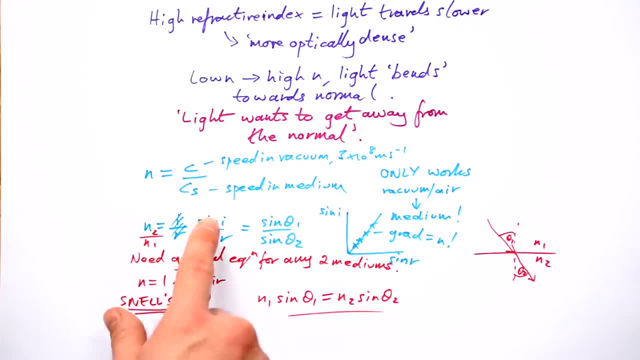 So if I was to incorporate this refractive index into this equation and for it to still be true, the only way I could do that is to divide the refractive index of this medium by one. So we've just figured out Snell's law. 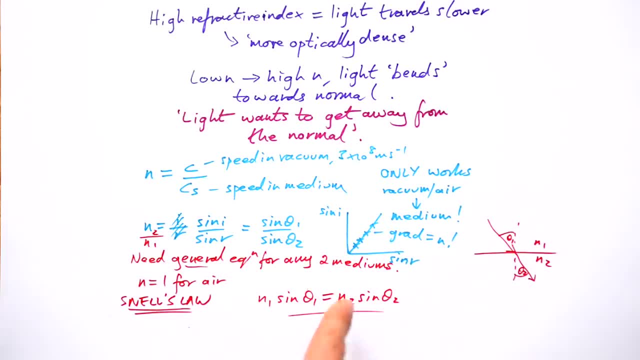 That is N one sine theta one. that's the refractive index of the first medium times. the sine of the angle of incidence equals N two: refractive index of the second medium times sine theta two. that's the angle of refraction. 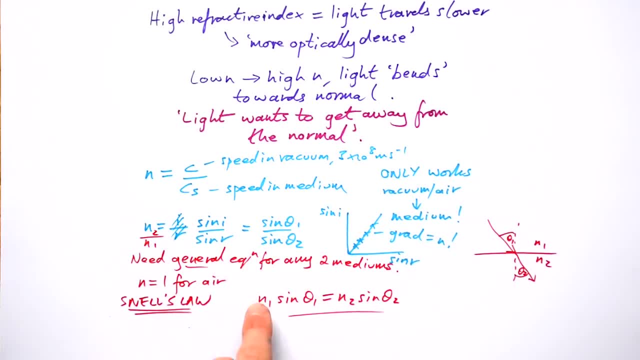 that's the angle after it's crossed the boundary. You could get given three of these things and be asked to find out a fourth. If it's to find the refractive index, all you need to do is rearrange to solve for that. 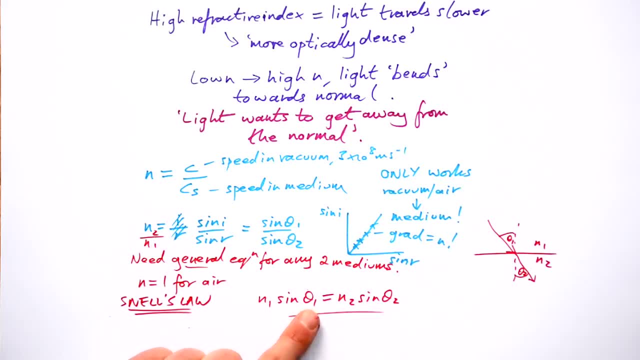 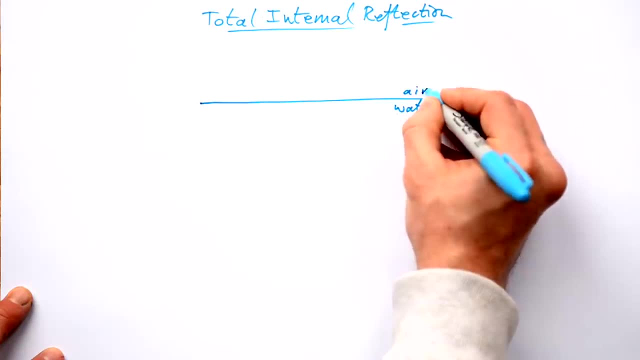 to make it the subject. If it's an angle, then you need to rearrange and then do the inverse sine of what you've got to find out the angle. Now let's say: we've got some water here, We have some air here. 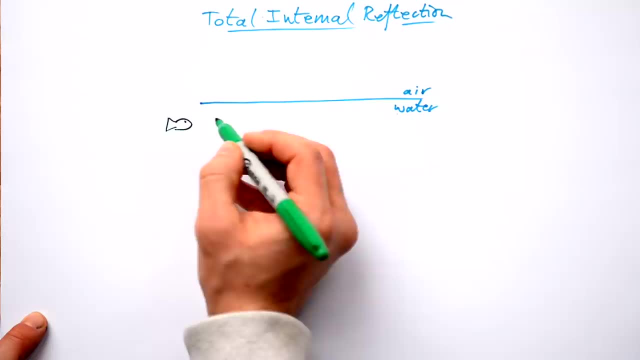 Now, if you were a fish down here and you could spit water up- and you do have these fish- there's a little bug on there and you want to spit some water up and take it down. You know that if light or if it's just water, that's no big deal. 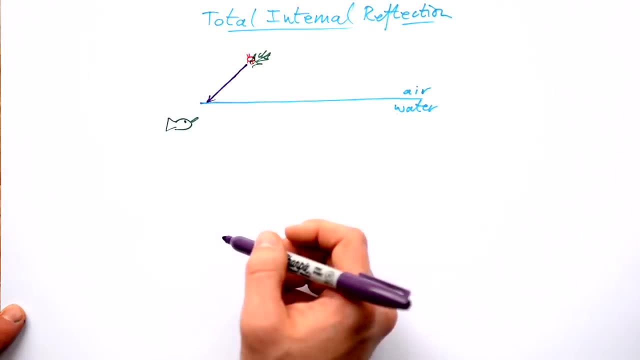 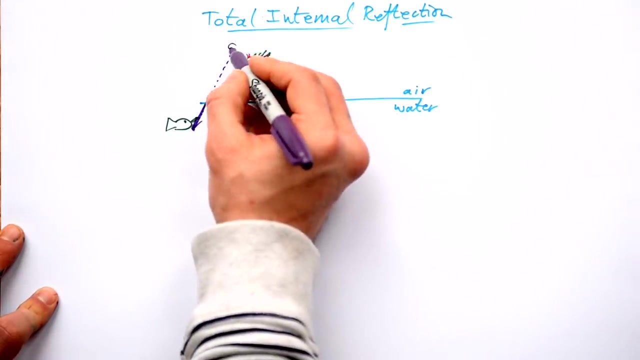 comes from this bug. When it hits the water, is it going to bend towards or away from the normal? Well, it's going into a more optically dense medium, so it's going to bend towards the normal like this. Now, if this is the light that's reaching the fish here, the fish sees the bug over. 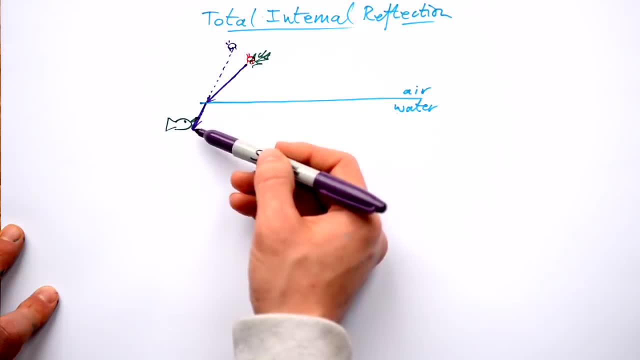 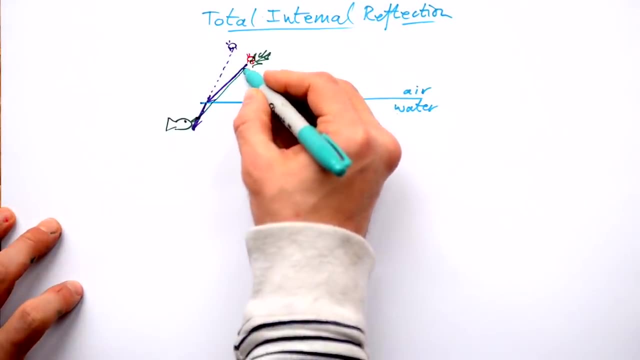 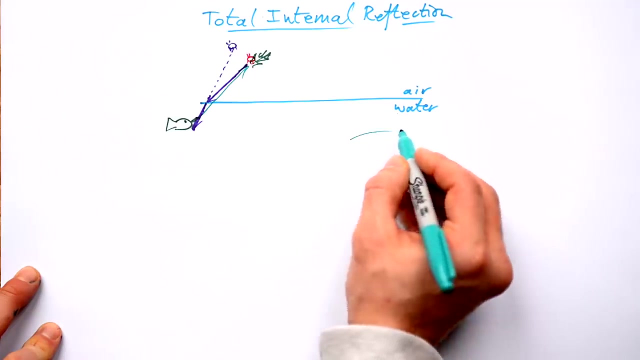 here, because our eyes, and fish's eyes, think that light travels just in a straight line, like that. What's really clever about these things, though, is that they can actually compensate for it, and they know exactly where to shoot in order to compensate for that refraction of light. Now, if you were a shark over? 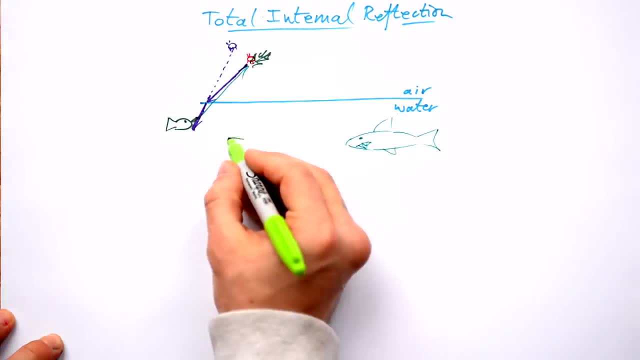 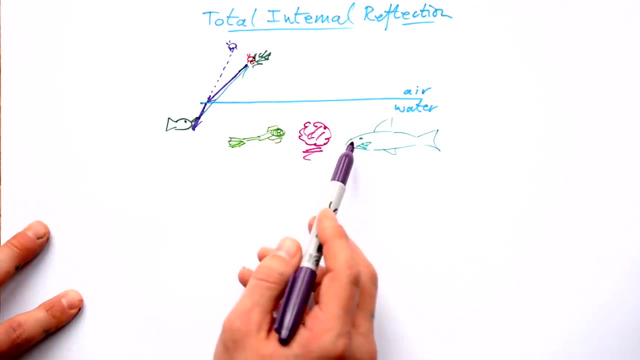 here and there was a scuba diver over here and there was some coral in between, so they can't see each other directly. Could the scuba diver see the shark with the reflection on the surface? Well, let's have a look. Light is coming from the 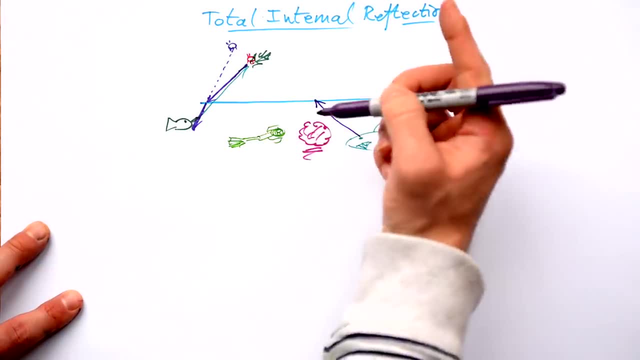 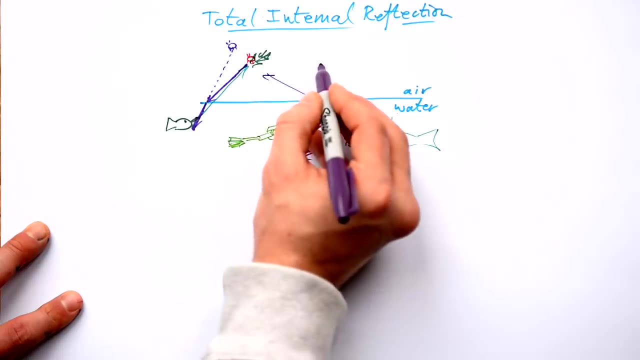 shark up to here. Now. light is going to be refracted so long as a specific condition is met And it's going to bend away from the normal, because we know light wants to get away from the normal. But you might not know that we always get a. 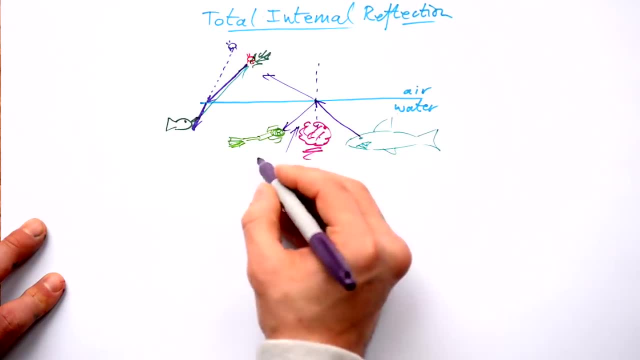 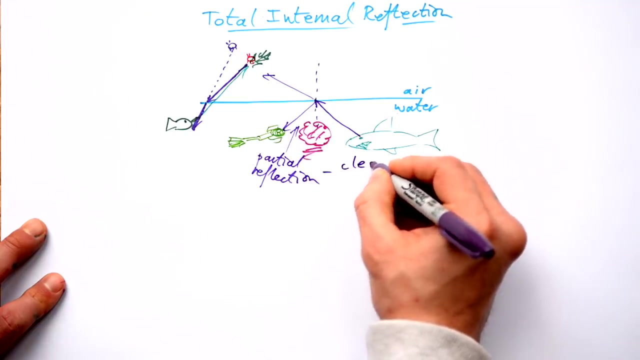 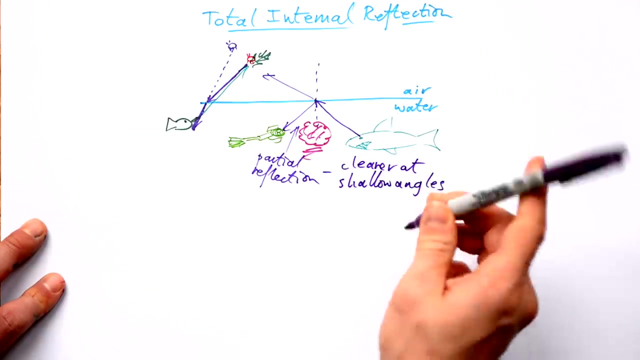 partial reflection as well. We always get a partial reflection. Most of the light is going to go out here, but some of the light is going to just bounce off. Partial reflection gets clearer or gets more at a shallower angle. If the light was coming in here instead, then we'd get more of a partial. 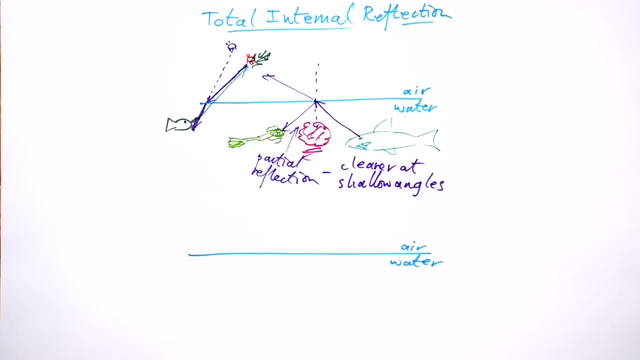 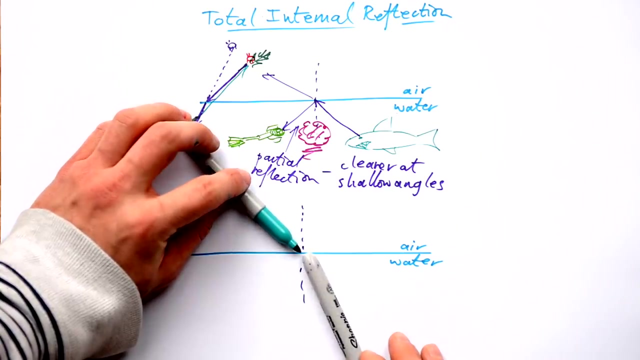 reflection. But we're going to forget about the partial reflection for now and we're just going to be looking at what happens when the angle gets really, really shallow. That's the angle between the boundary. So if light comes in like this from air into water, then that means the light ray bends towards the normal. 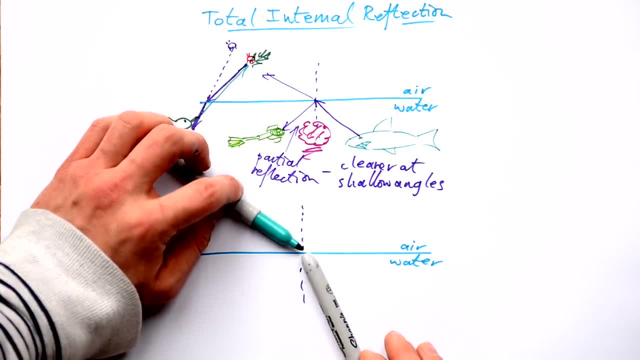 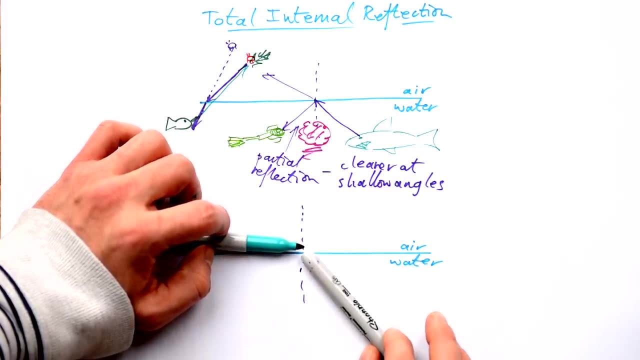 like that? What if we increase the angle of incidence round like that? Well, the angle of refraction would increase. but eventually we're going to reach a limit with our angle of refraction, aren't we? We're going to hit 90 degrees. At that point, light can't be refracted anymore. 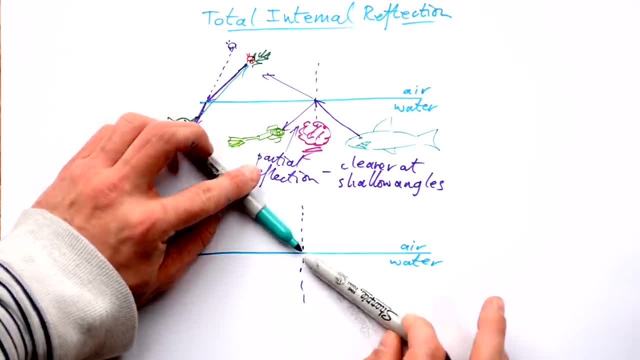 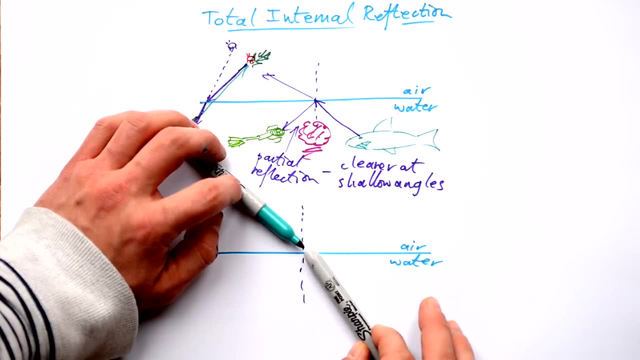 We've reached a maximum angle of refraction, But the point is, whenever light goes from a material with a low refractive index into a higher refractive index, like air and water, then it's always going to be refracted. However, what about if we do it the other way around? We 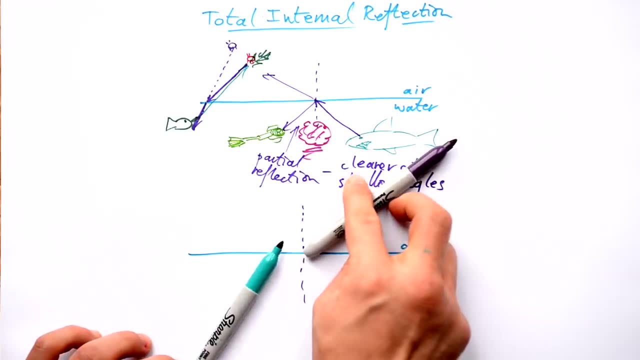 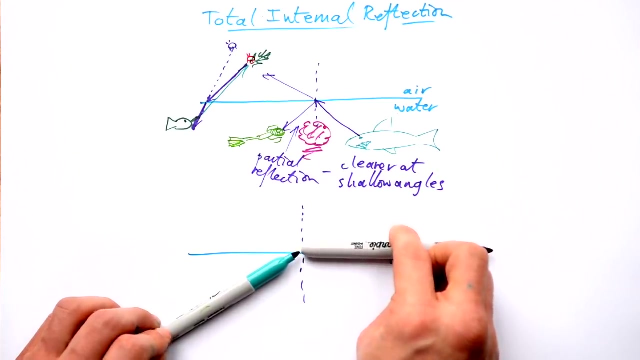 have light coming out of the water and going into the air, like so It's going to be bending away from the normal. What happens if we increase this angle of incidence, going from the bottom more and more and more? Eventually, this angle of refraction is going to reach 90 degrees, like that. This angle 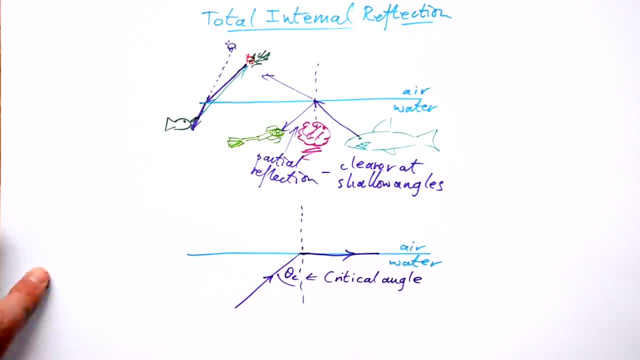 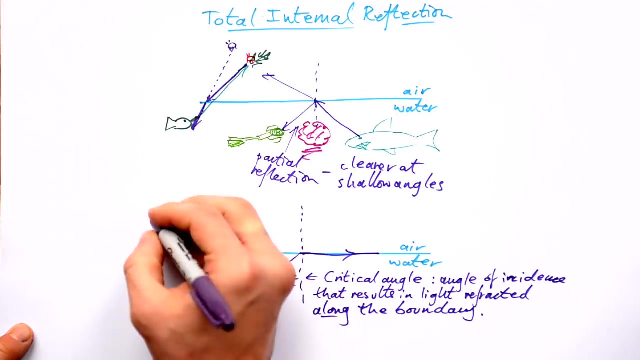 here is now called the critical angle. Critical angle is the angle of incidence that results in light refracted along the boundary. So for glass that's about 42 degrees. Let's go back to Snell's law real quick: N1 sine theta 1 equals N2 sine theta 2.. But in this case we know that our 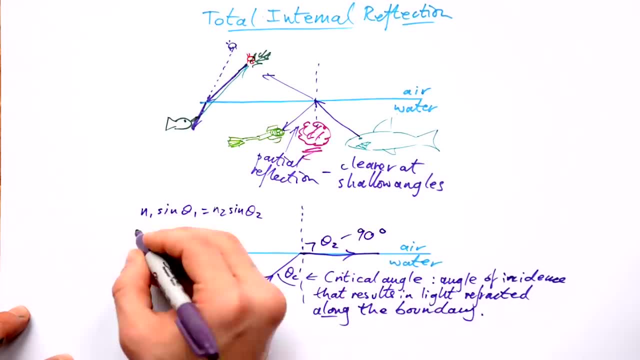 angle of refraction is going to be 90 degrees at this point. So we can say: N1 sine theta C- that's our critical angle- equals N2 sine theta 2- 90. Sine of 90 degrees is 1.. So we can just get rid of that. 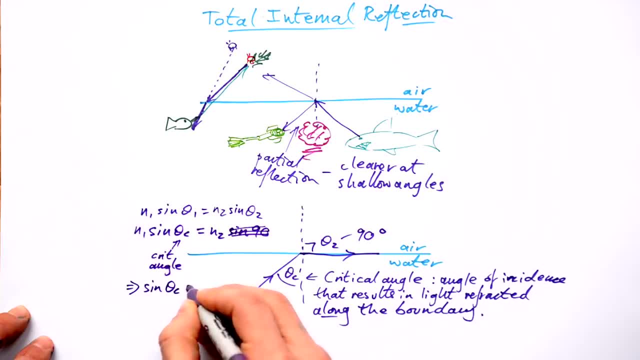 So we can figure out. the critical angle is equals the refractive index of the second medium divided by the refractive index of the first medium. Now, we saw earlier that we always have a little bit of a partial reflection, don't we? But what's gonna happen above this critical angle? no light is. 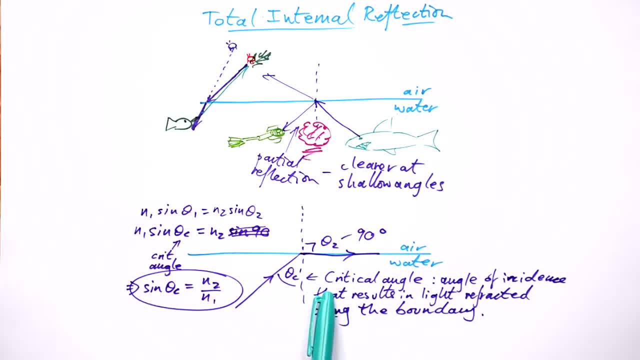 going to be refracted into the other medium. All of the light is going to be contained in the first medium, which means that all of the light is being reflected, hence the name total internal reflection. when theta 1 is greater than the critical angle, no light is refracted, all light reflected, and that is T? I, our total. 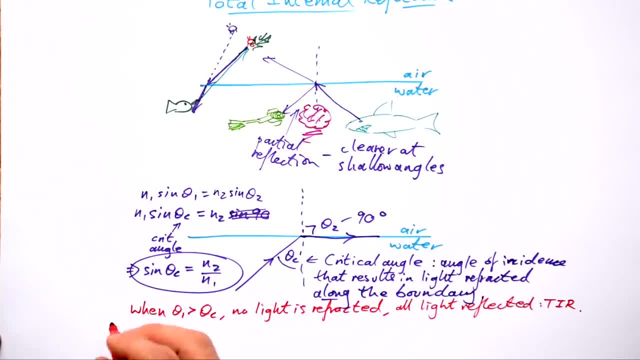 internal reflection. so you'll notice that we need two things to happen. for T IR to occur, two conditions needed. one, the light must be in the more dense medium. that means the higher refractive index, TIR, can't happen if light is going from air into water. it only goes from water into air. and the second condition: 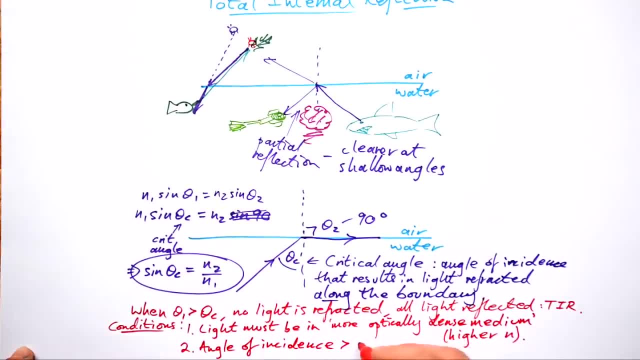 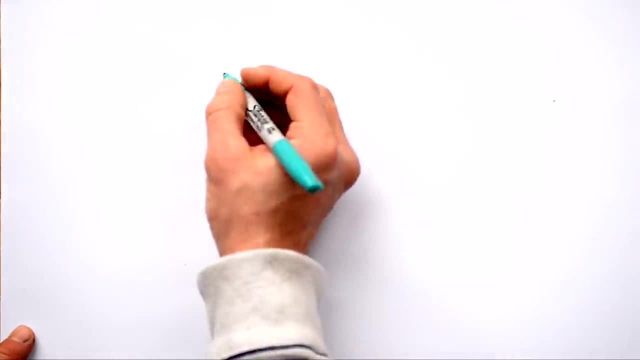 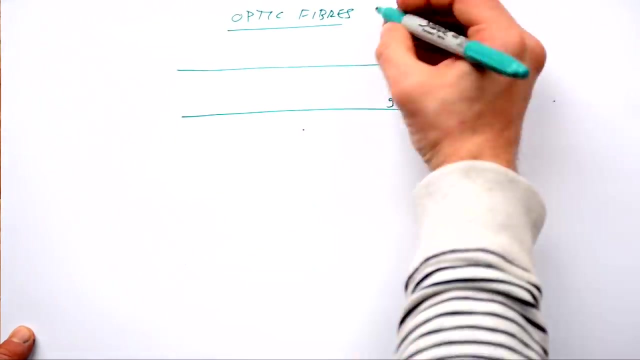 like we saw, angle of incidence has to be greater than a critical angle. so those are the two conditions that you need to remember that result in total internal reflection happening. so what is the point of TIR? how can we use it in real life when you use it with fiber optic cables- gonna call that optic fibers sometimes- you'll. 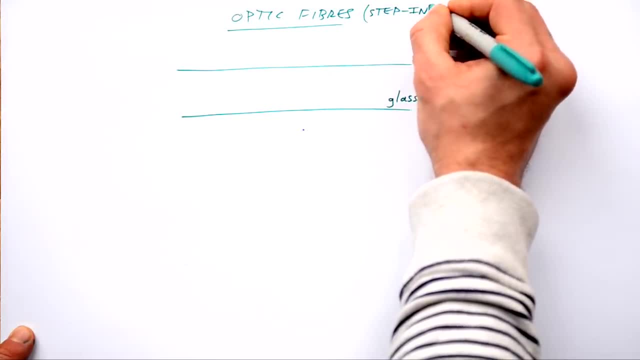 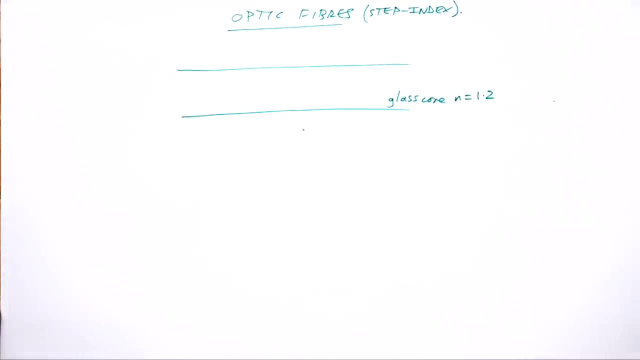 see these referred to as step index. I'll talk about why you might call them that in a second. so let's say that this glass core has a refractive index of 1.2. these glass fibers are very, very small. if it was just air outside which has a. 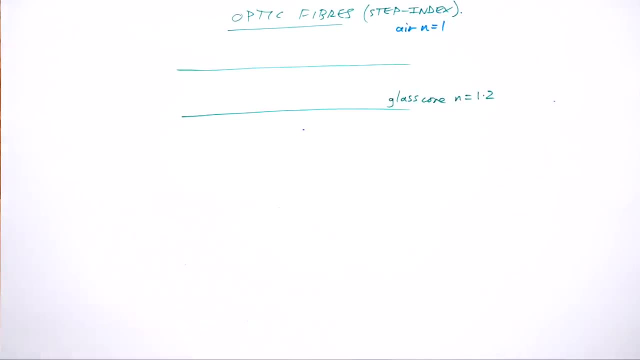 refractive index of one, then TIR is going to be greater than the critical angle TIR could happen when the light comes in at a shallower enough angle. then it's going to bounce off like that because it's in the medium with the higher refractive index. problem is: it's not a good idea to just have a fiber optic. 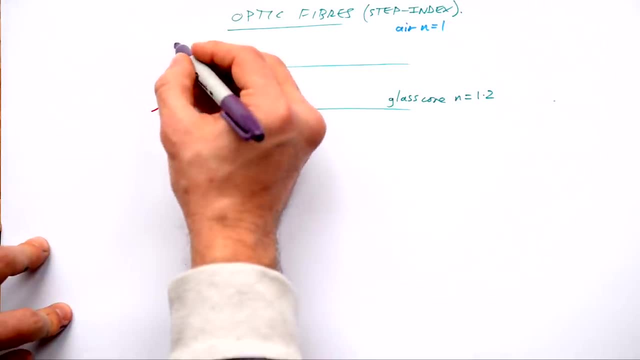 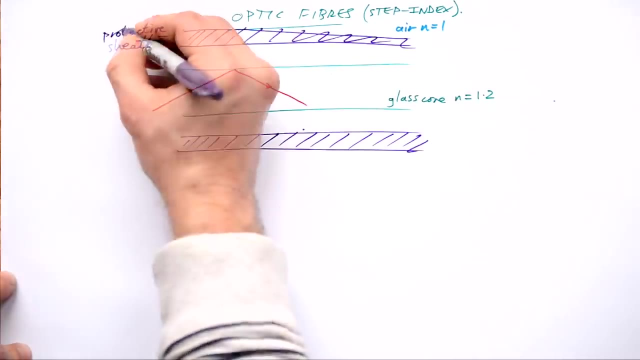 cable, just the optic fiber, the glass bit. generally we have protective casings. we call this the protective sheath. now this is going to have a very high refractive index. so let's say it's going to be n equals 1.8 or something like that. it's going to just be. 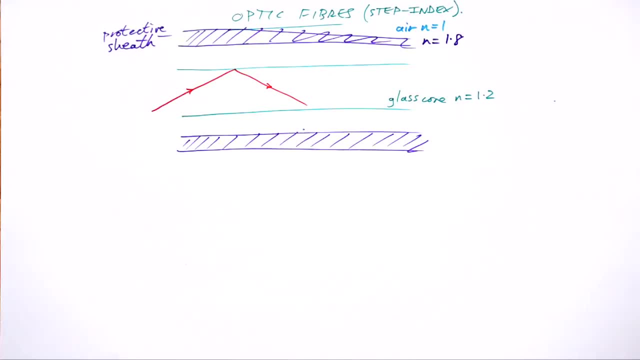 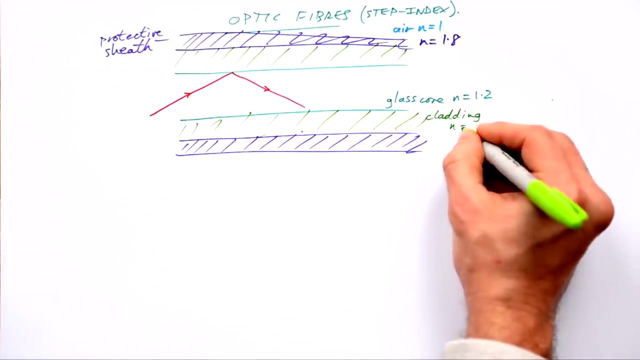 plastic, isn't it? so the problem is, if this sheath was touching the glass core, then it would be impossible for TIR to happen, so we need something in between. so what we have is this special cladding around the outside, and this has a lower refractive index than the glass core, which means 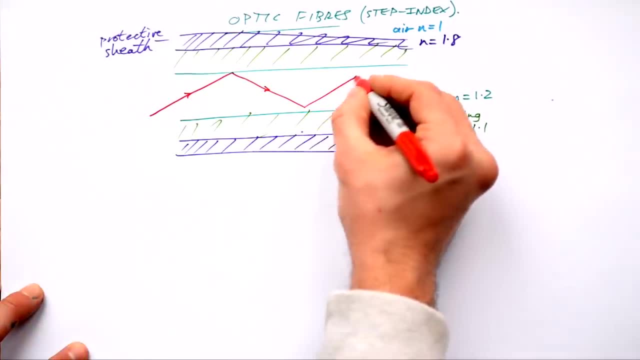 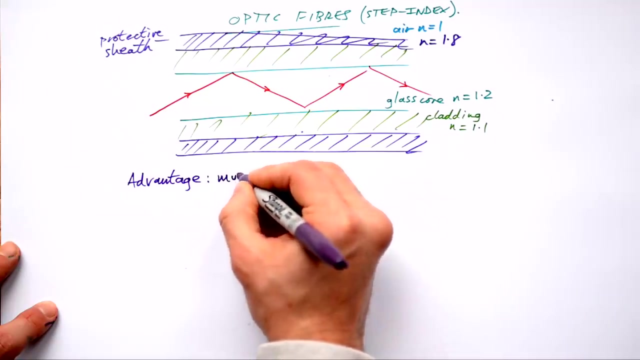 that TIR can happen. that's what happens. light goes along. this fiber optic cable gets sent by a transmitter, received by a receiver, and that's a way that you can send information very quickly. an advantage to fiber optic cables is that you can multiplex. that means sending different frequencies. 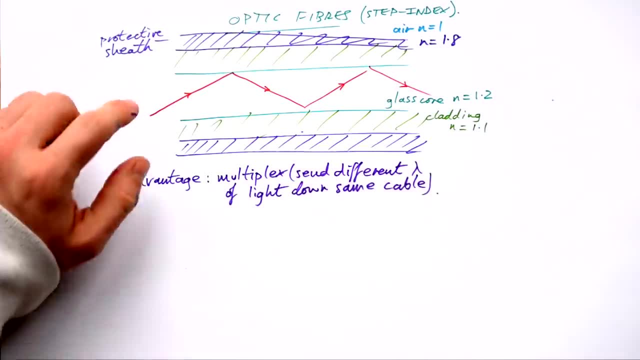 different wavelengths of light down the same cable, so you could send red light, green light to blue light, as it were, down this same cable and they wouldn't interfere with each other, and then they could all be picked up at the other end. now, when we send light down, we do get a little bit of